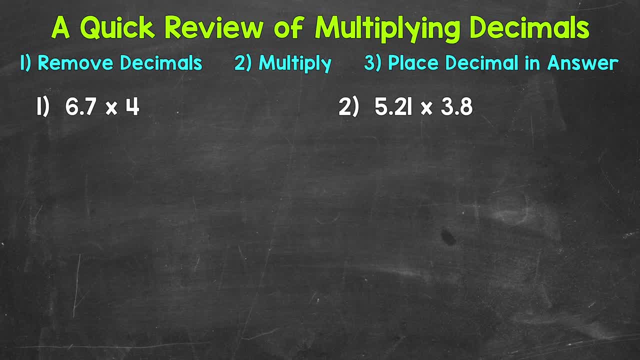 really no matter what class or goal you are working towards. here are a couple of examples to get this down. Let's jump into number one, where we have 6 and 7 tenths times 4.. Now the first thing that we're going to do when we have a multiplication problem. 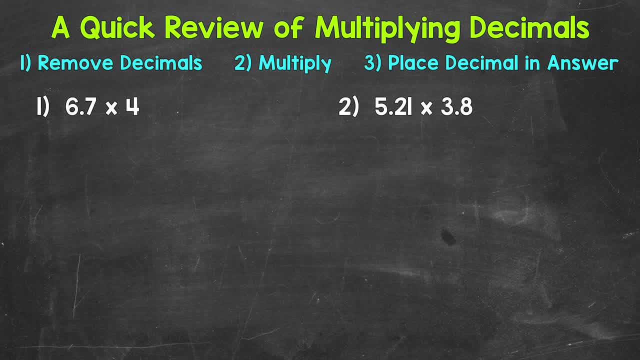 that involves decimals. we're going to remove any decimals within the problem. So we're going to multiply just like we would if we had whole numbers. Let's set this up and rewrite number one as 67 times 4.. So, again, remove any decimals. We're going to worry about placing the decimal in our answer. 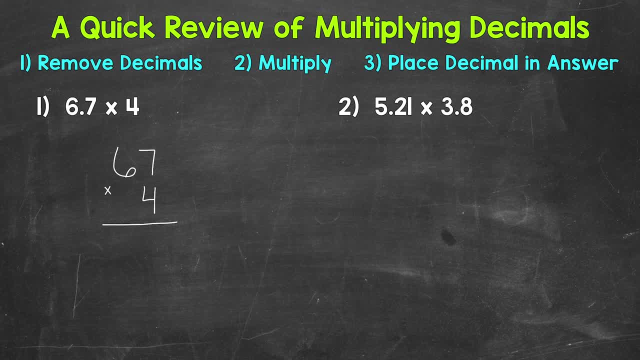 once we multiply. So once we remove the decimals, we can multiply. So we'll start with 4 times 7,, which is 28.. So carry that 2.. And then we have 4 times 6, which is 24,. plus that 2 is 26.. 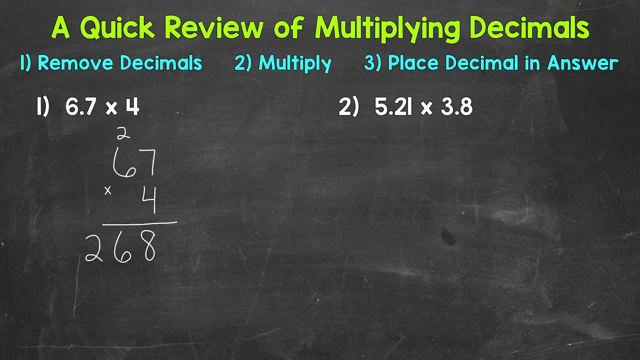 Now we're done multiplying So we can place our decimal in our answer. So we take a look at the original problem and see how many digits are behind or are to the right of a decimal. Well, 1. We have this 7 right here, to the right of a decimal. So our answer is going to have: 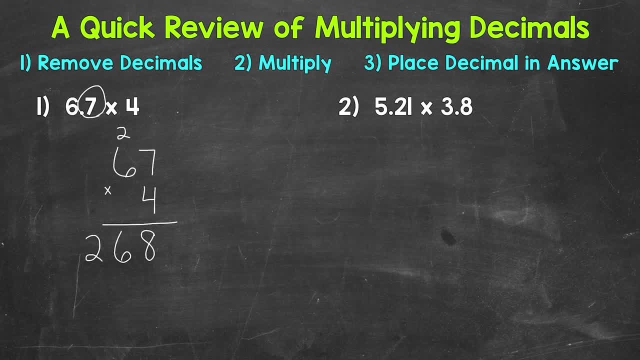 one digit to the right or behind the decimal. So one digit would be this 8, so we can place our decimal in between the 6 and the 8.. Our final answer: 26 and 8 tenths. Let's move on to number two, where we have 5 and 21 hundredths times 3 and 8 tenths. So 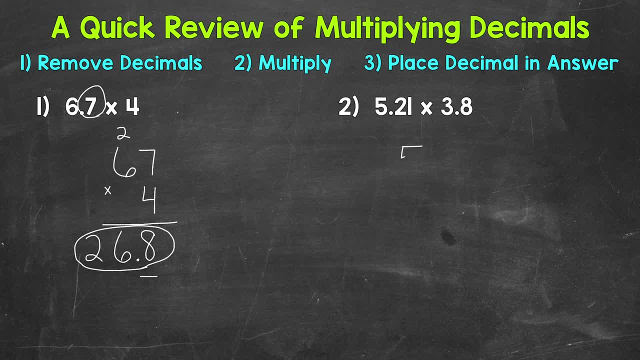 let's remove the decimals and rewrite this problem. So 521 times 38.. Now we're ready to multiply. So 8 times 1 is 8.. 8 times 2 is 16.. Put our 6, carry the 1.. 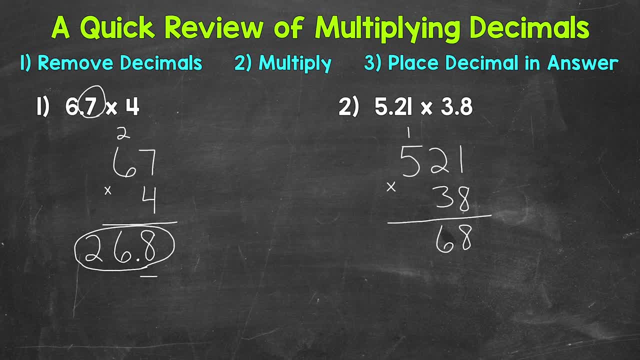 And then 8 times 5 is 40, plus that 1 is 41. So we are done with the 8, and we are done with this carried 1.. So we're going to move over to the 3.. We're moving one place value to the left.